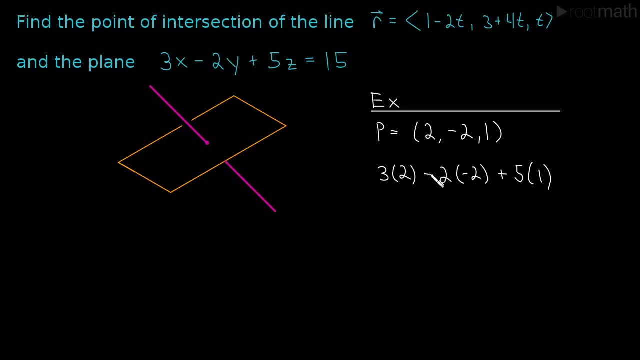 Okay, and this is 6 minus, or sorry. 6 plus 4 is 10, plus 5.. This is 15.. So that checks out. This is a point in the plane, because when I plug it in and do this addition and multiplication- 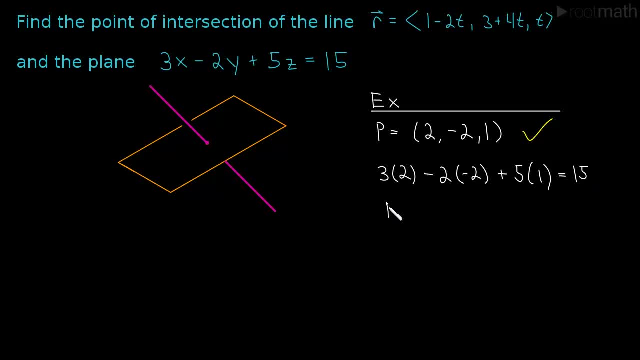 I end up with the number 15. So here, real quick, is a non-example. So the point Q equals 1, 1, 2 is not a point in the plane, Why? Because when I plug that in I get 3 times 1, minus 2 times 1, plus 5 times 2.. 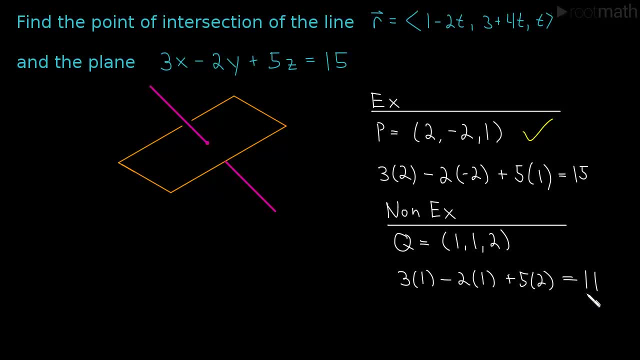 This simplifies to 11, which obviously, of course, is not 15.. So this is not a point in the plane, because when I plug it in, I get 11 instead of 15.. Okay, so we have this really basic concept. 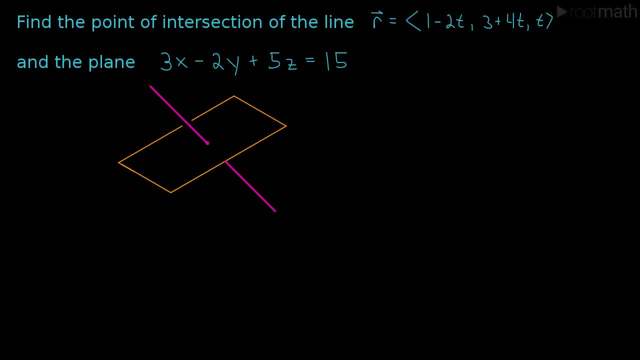 We spend about two minutes discovering what it means to be a point in the plane or kind of rethinking about that. Hopefully you already knew it, And so if I come up here, let's think about what it means to be a point on the line. 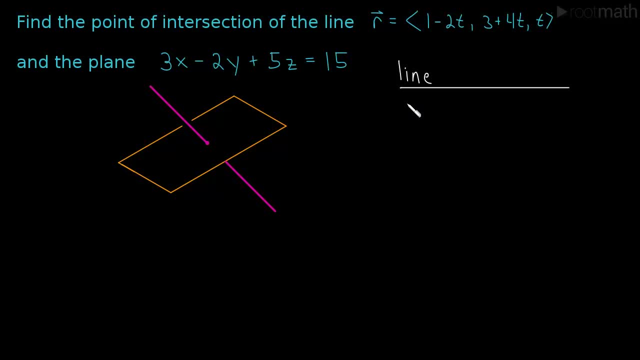 So here this is the vector equation of the line, but I could write out the parametric equations, And this is just telling me that x is 1 minus 2t, y is 3 plus 4t And z is just t. 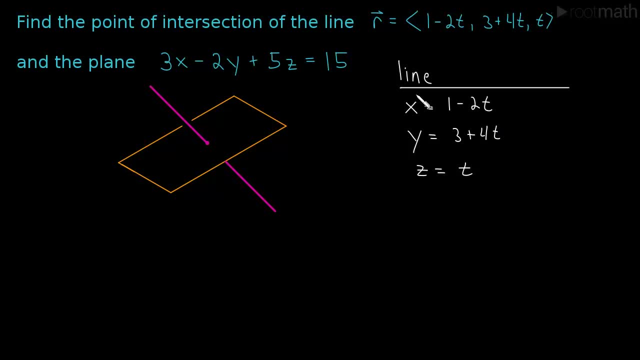 So if I plug in any t value, what I get out is a point. I get the x, y and z coordinates of a point on the line. So this gives me a point on the line and I want it to be not only just a point on the line. 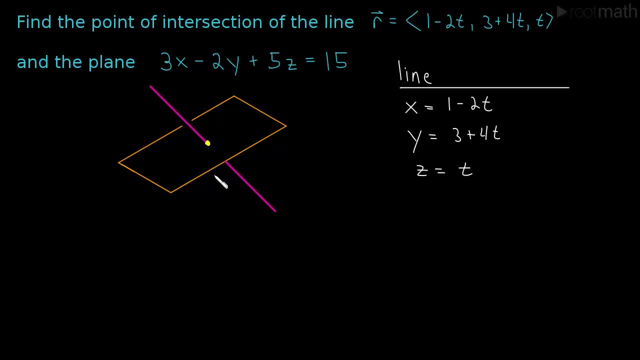 but also a point in the plane. That's what it means to be an intersection point. You're a point on the line and you're a point on the plane. Oops, Didn't mean to do that, But we've already just talked about what it means to be a point on the plane. 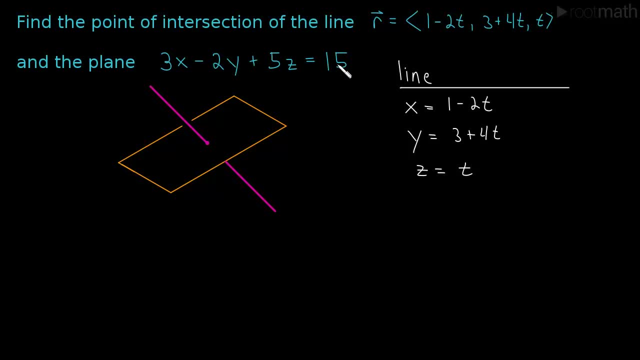 It means when you plug in into this, you're equal to 15.. So what that means is, if this is a point on the line, this is a point x, y, z. it's giving us a point And we want to make sure that's on the plane. 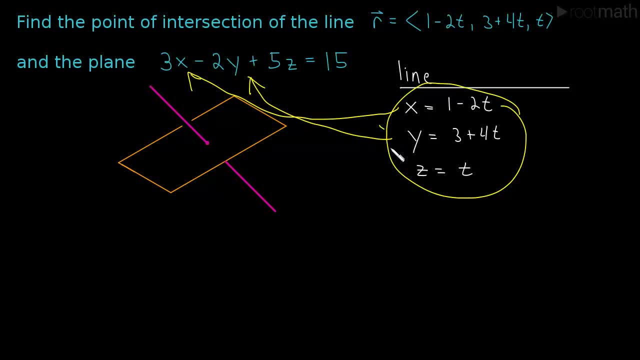 We should just plug in x in for x, y in for y and z in for z and make sure that it's equal to 15.. Okay, So all right, enough discussion, Let's actually do the computation here. So what do we have to do? 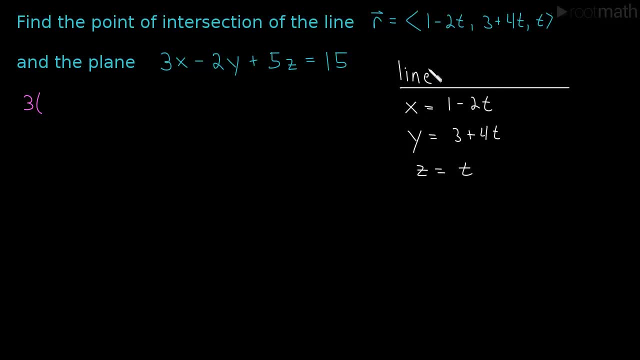 We take the x here. This is a point on the line, remember, and we're plugging it in to see if it's going to be a point on the plane. So in for x goes 1 minus 2t minus 2, and then we plug in y, which is 3 plus 4t plus 5,. 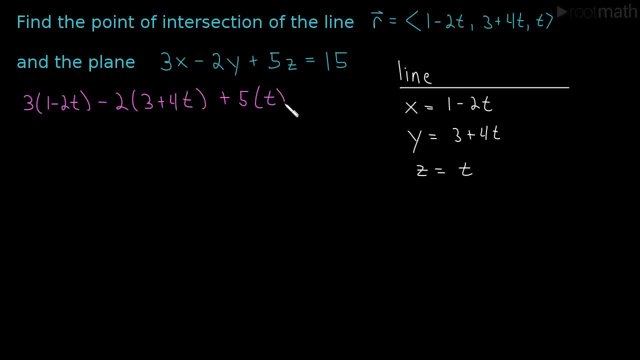 and then we plug in t And for z and we want to. what's happening is we're saying we're plugging this in and we want to make sure that this is equal to 15.. Okay, Let's simplify this a little bit. 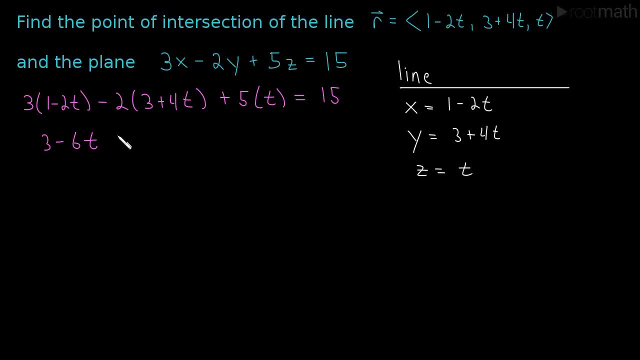 This is 3 minus 6t, and then minus 2 minus 8t plus 5t is equal to 15.. And now, oops, I wrote something down wrong right here. This should be minus 6.. So I distribute this minus 2 to the 3.. 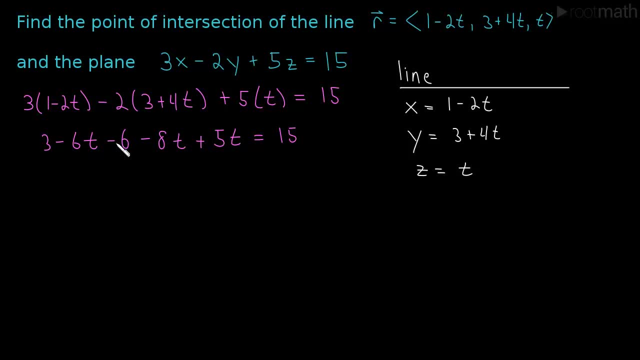 That should be a minus 6 there, And so the constant on this side is 3 minus 6, so that's minus 3.. So we can add that over We'll get 18 on this side, And then minus 6 minus 8 is minus 14t. plus 5t is minus 9t. 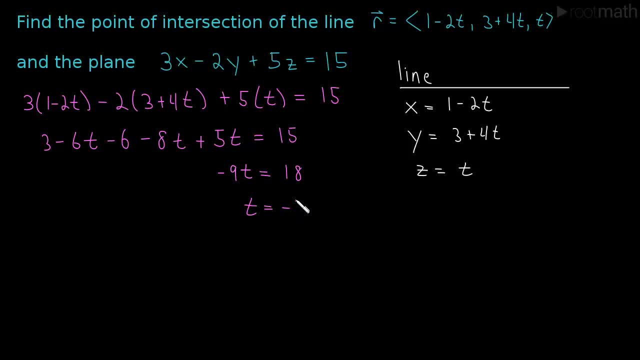 Divide by minus 9, and we get 15.. t is equal to minus 2.. Okay, So what did we figure out? We were looking for a point of intersection and all of a sudden, we kind of went through this analysis and we ended up with t equals minus 2.. 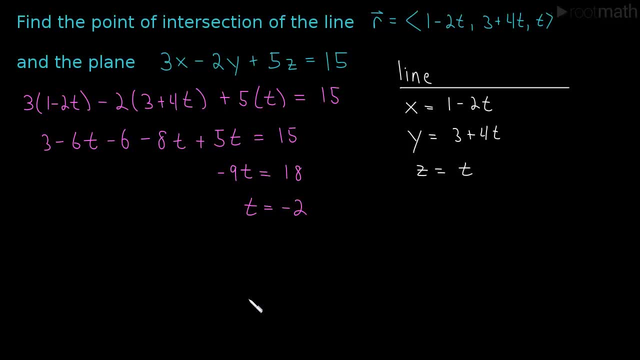 Well, that's certainly not a point. It's just a t value, But it is, it does have some significance. So let me take this computation. We all it, or what it helped us figure out, was that t is equal to minus 2.. 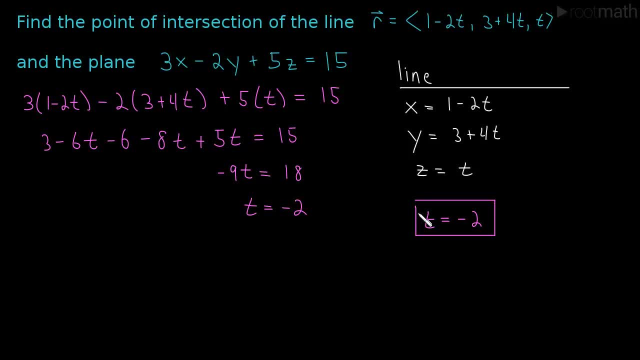 And what does this mean? What is this? t equals minus 2? Well, it tells us how to find the point Because, remember, what we said is we could plug in any t value. It will give us a point on the line. 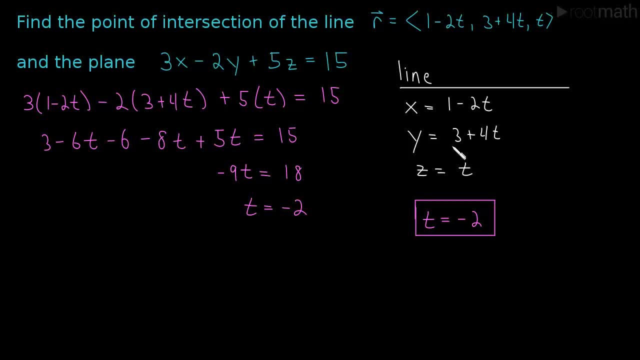 And what this is saying is: you plug in this t value, it will give you the point on the line. that is also the point in the plane. That was the whole point of this computation. When t is minus 2, the point that comes out will be a point in the plane. 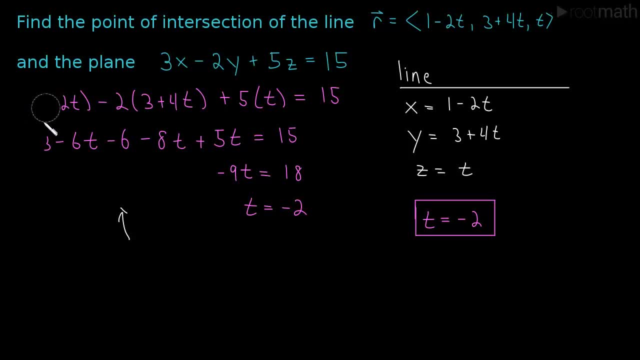 Okay, So let's, let's continue on here. We're almost done. So the point on the line- or, sorry, the point we're looking for, then, is the point that says plug t equals minus 2 into this, this equation for the line. 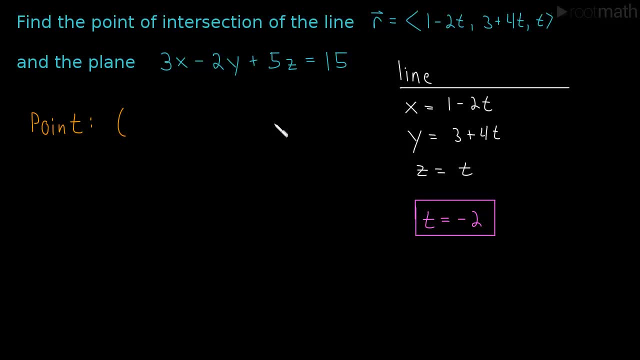 And what point comes out? Well, the, the x coordinate is 1 minus 2 times the t value, which is minus 2.. The y coordinate is 3 plus 4 times minus 2.. And the z coordinate is just minus 2, goes in for t. 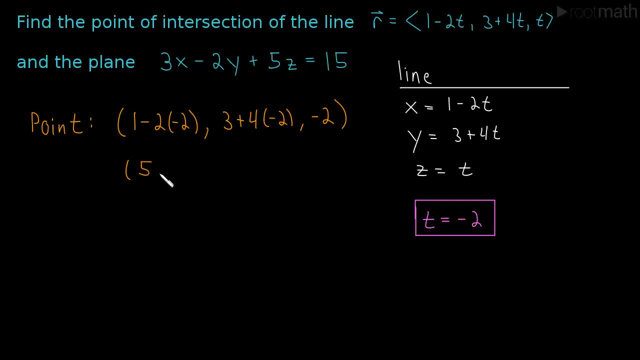 And so let's simplify this a little bit. This is the point: 5 minus 5, minus 2.. So this is certainly a point on the line. I mean, that's where it came from. We plugged minus 2 into the line. 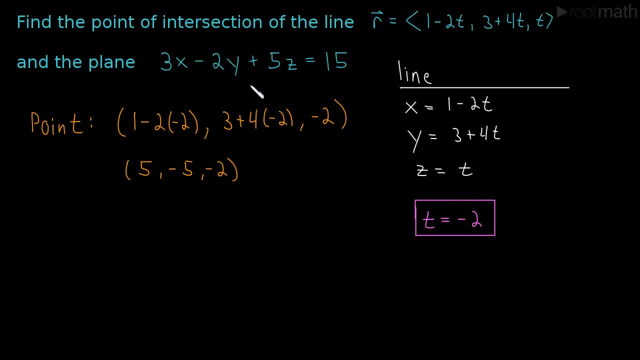 And because we got this t value by plugging the point into the equation for the line, we're guaranteed that this is actually a point in the plane also. But let's just go ahead one last, do one last check here And check that that actually is a point in the plane. 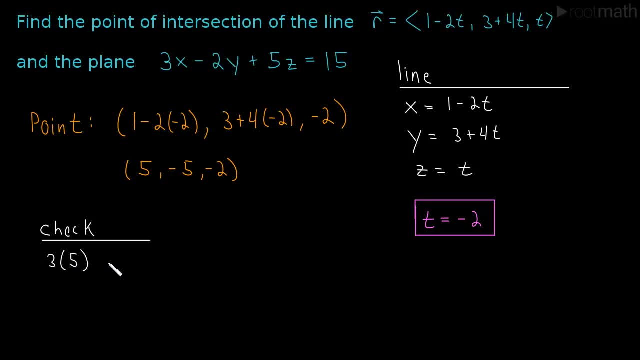 So we do 3 times the x coordinate of our point, which is 5.. Minus 2 times the y coordinate, which is minus 5.. Plus 5 times the z coordinate, which is minus 2.. And this becomes 15 plus 10, minus 10, which just simplifies to 15..